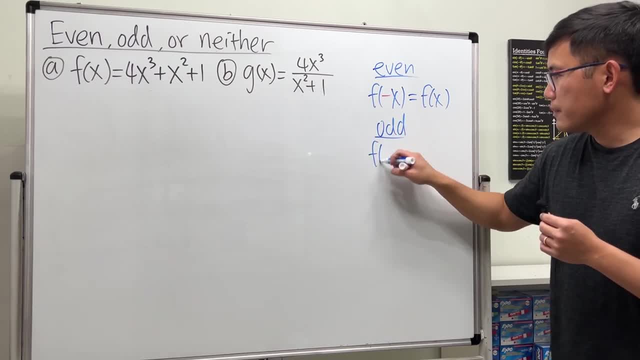 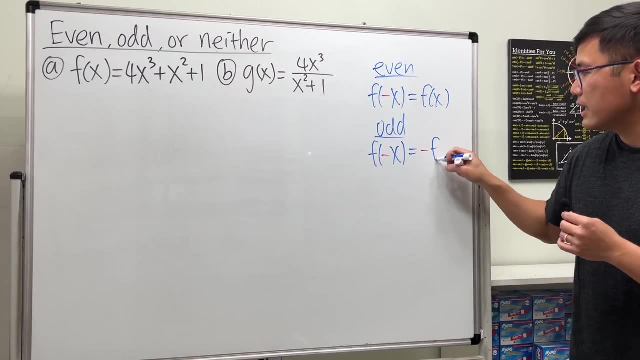 If a function is odd and again we plug in negative into the function here, If this negative stays and we can factor that on our side like this, then the function is odd And this right here will give you a 180-degree rotation. 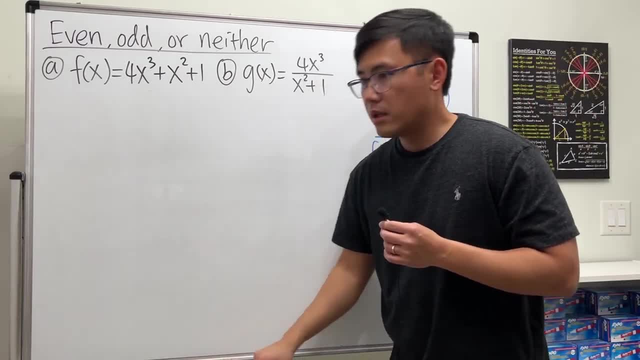 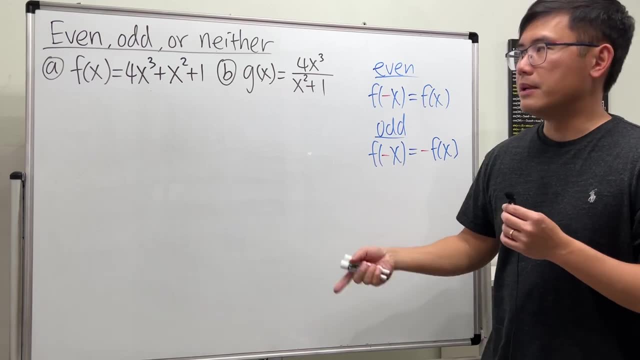 And then the graph will be even And the graph was still the same. That's what it means: to have a function that's symmetrical about the origin. So either way, we have to compute this and see what happens. So let's go ahead and just get started with the first one here. 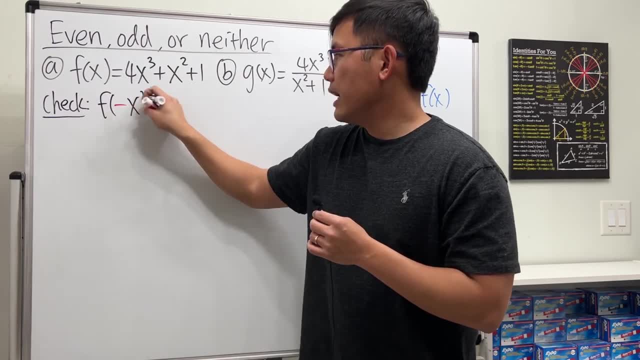 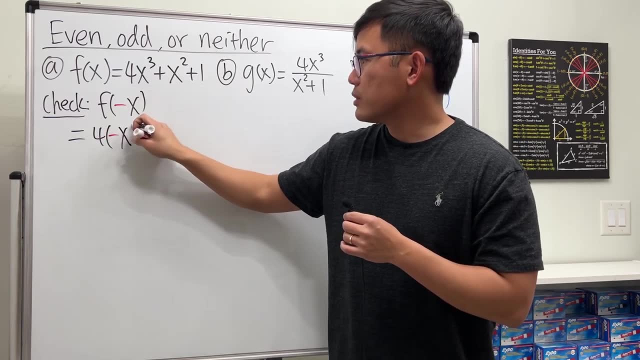 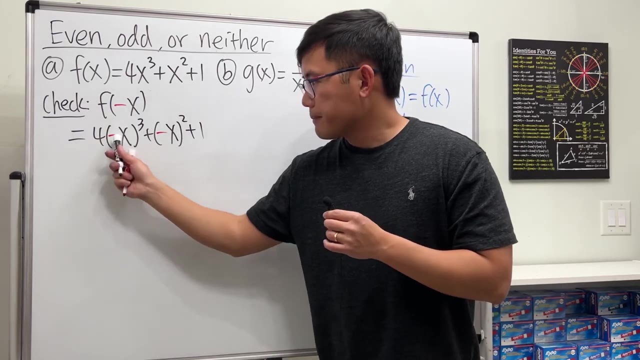 We check f of negative x And that just means that we plug in negative x into here and here. So 4 times negative x to the third power plus negative x, and then square plus 1.. Okay, this is pretty much negative 1 raised to the third power. we still get negative 1.. 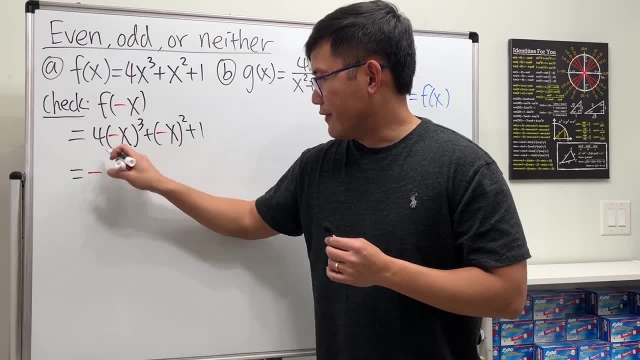 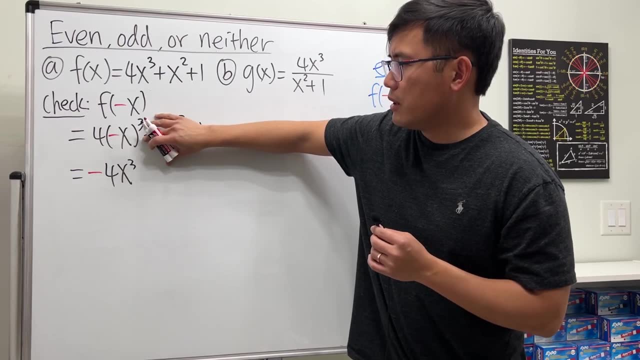 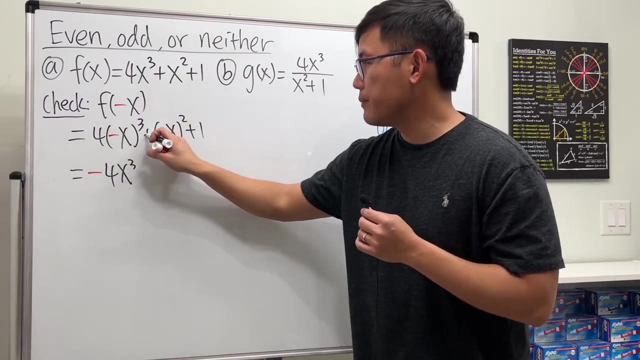 So the negative stays for the first part, And then we have 4 and then x to the third power. Therefore, if you just look at the first term here, that part by itself will have been odd. By itself it would be odd, but we still have to consider the other ones. 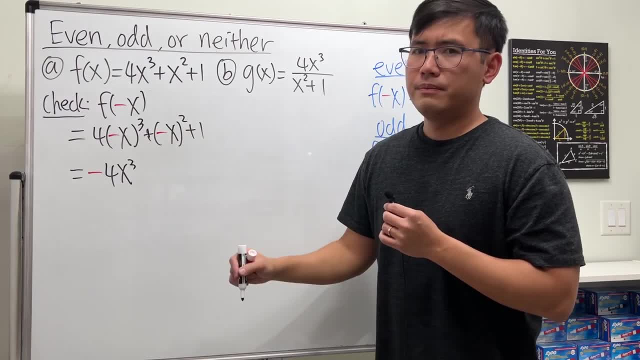 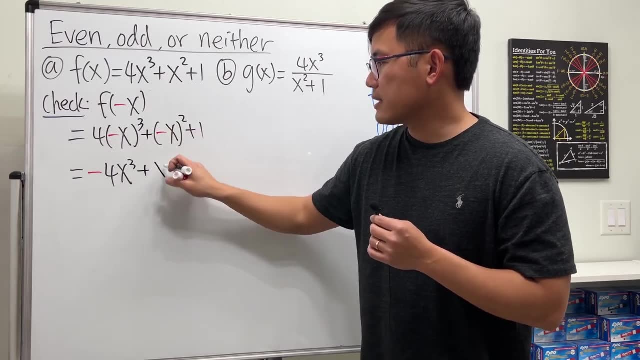 For the other ones this right here: negative 1 squared is positive 1.. So the negative disappears. So for the second term we have positive x squared And then the plus 1 is just plus 1, like this Hmm. 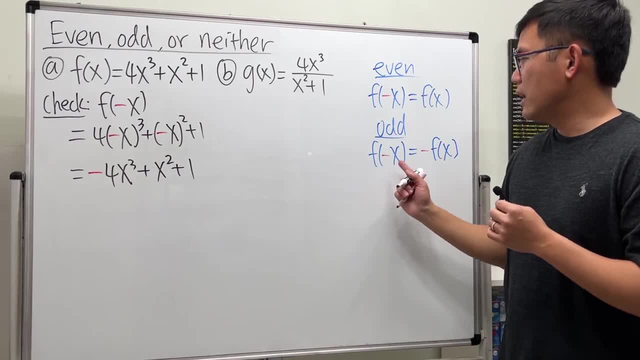 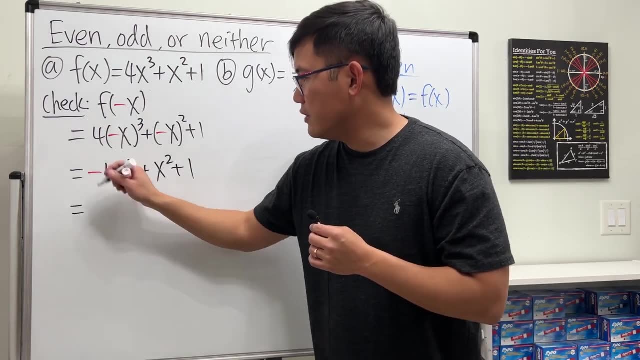 We have a negative all the way at the front, so does that mean we have an odd function? Is this the same as that? No, Because if you want to factor out a negative, then this would be negative times and this right here would be 4x to the third power. 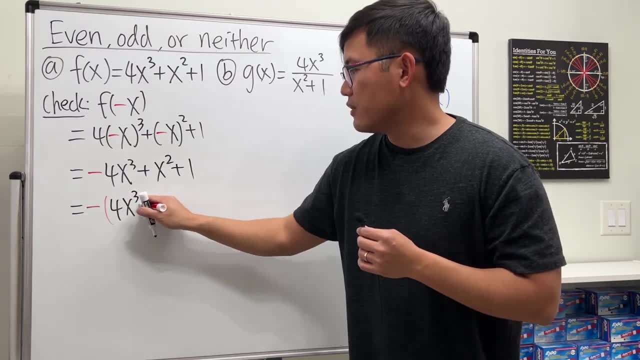 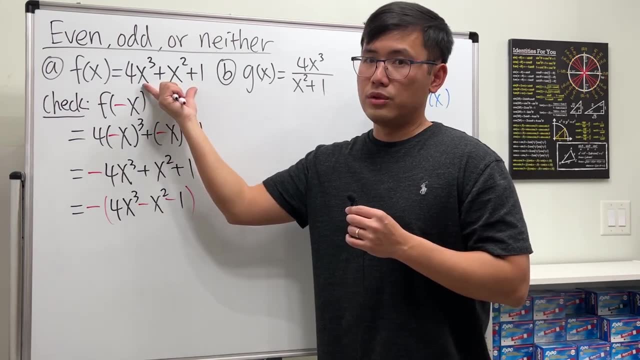 Remember, We would have to change the sign if you factor out a negative And then also change the sign here. This is no longer the same as the original. It looks like it, though, but it's not Be really careful. So be really careful. 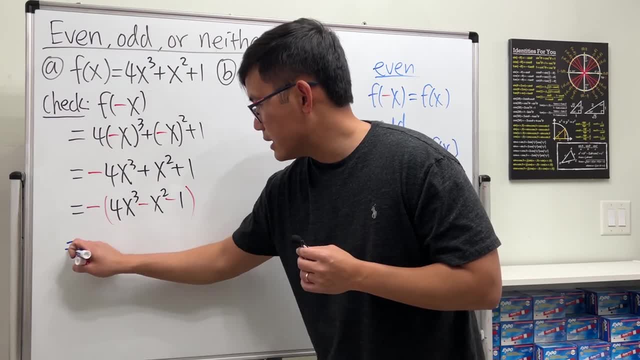 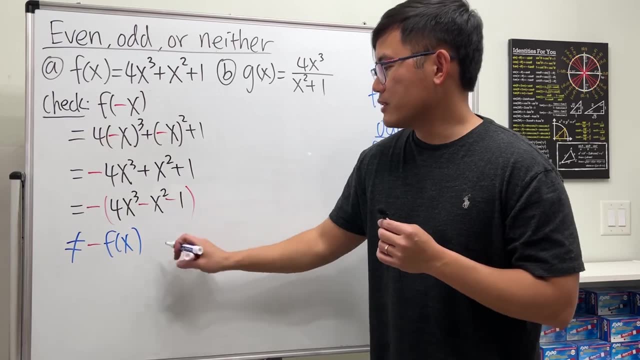 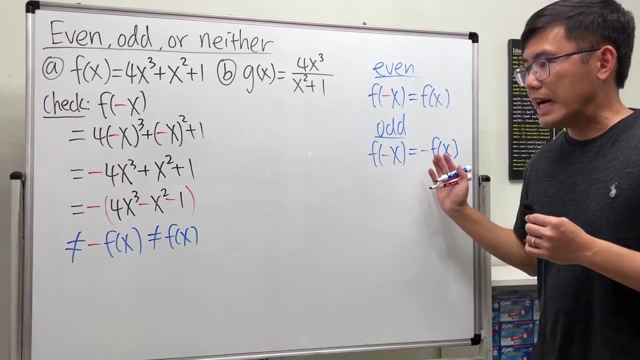 This right here is actually not the same as negative f of x, And because we have the negative, we can also say that this right here is not the same as just the original Right. This is not the same as negative f of x, so it's not odd. 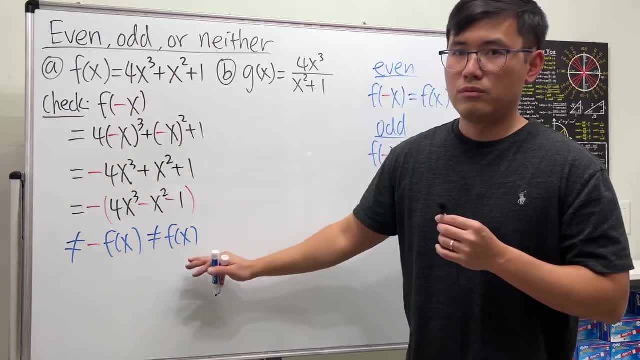 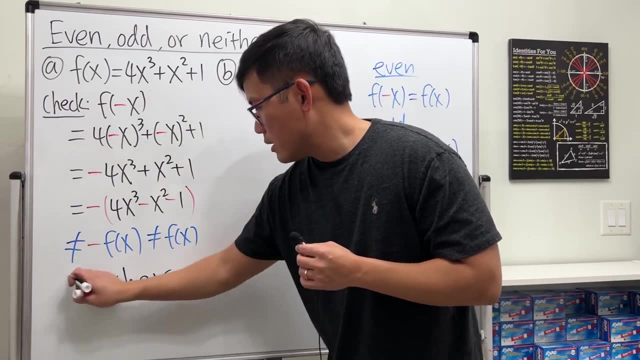 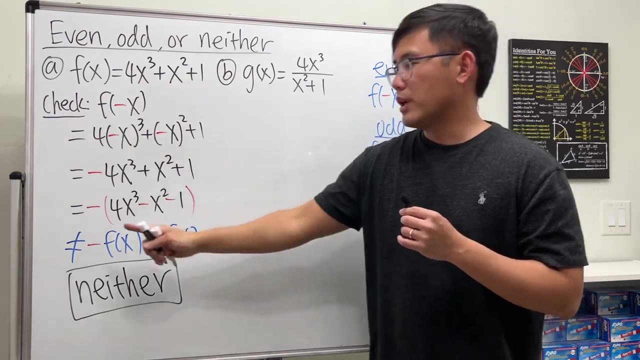 And this is also not the same as the original, so it's not even. Therefore, this right here is neither. So don't let this negative sign trick you. all right, Even though this part in black is also the same as the original. but we have to do it carefully. 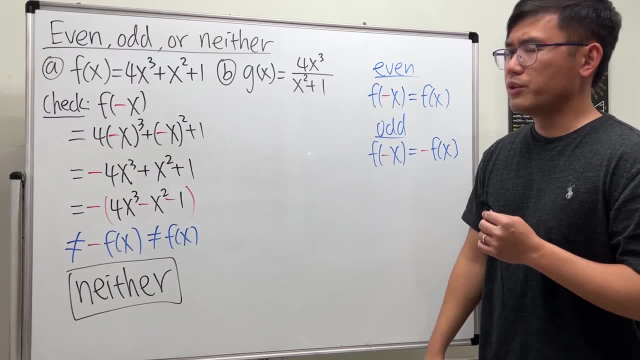 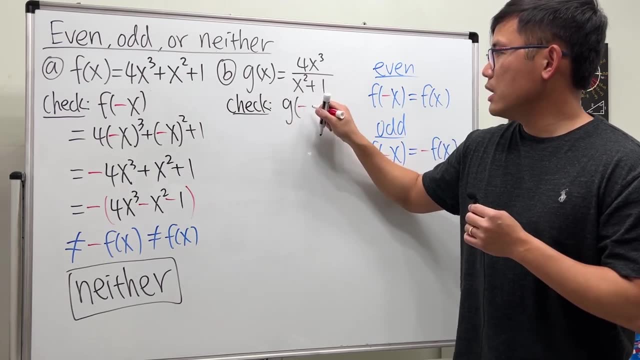 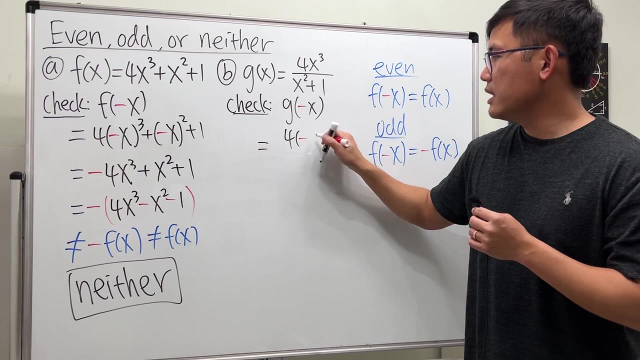 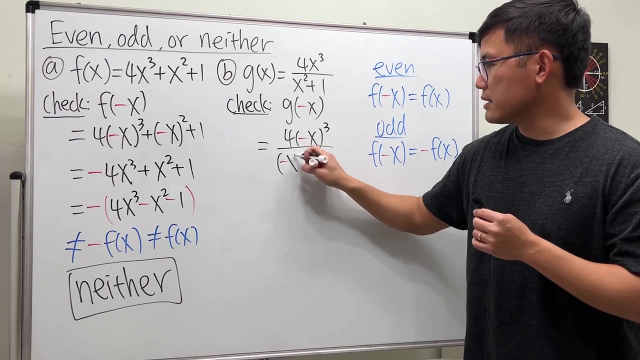 So does that mean for the second one it's also neither. Well, check this out Again. We do the same check. We plug in g, We plug in negative x into g like this, and in this case we will get 4 times negative x and then to the third power over negative x in here. so negative x squared plus 1.. 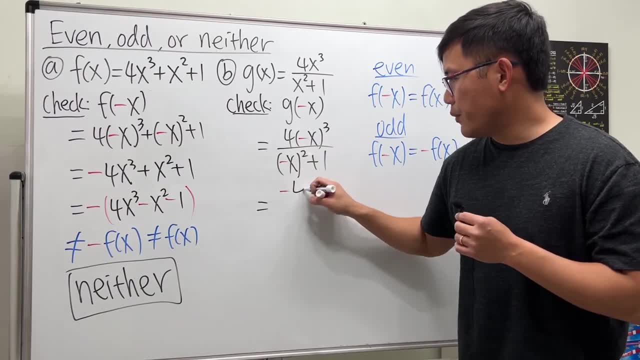 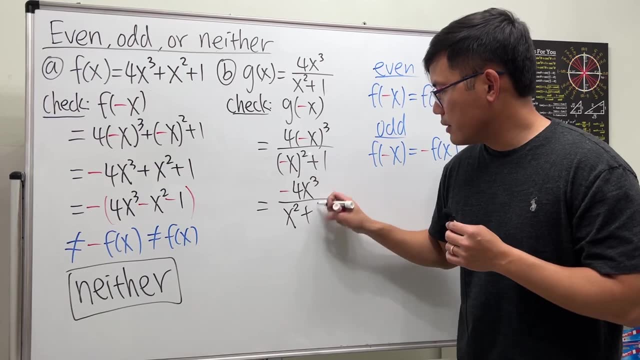 Negative 1 to the third power- we have a negative right here- and then 4x to the third power over This right here. is true, It's just x squared, and then plus 1.. Okay, But in this case, have a look. 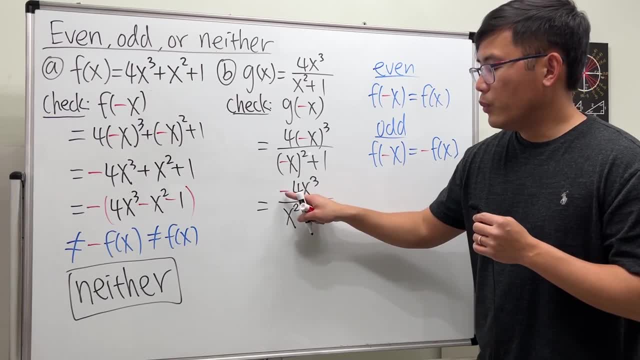 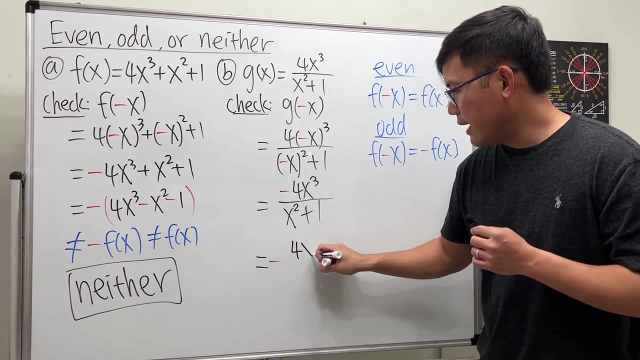 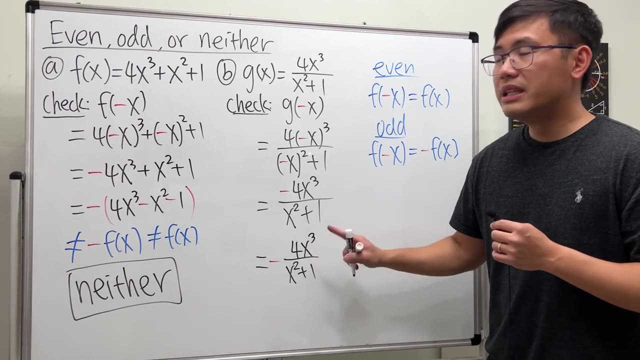 Negative 4x to the third power. we can put a negative to the front, nice and easy like this, and then this part will stay: 4x to the third power over x squared plus 1.. And if you look at this part, this is the same as the original. 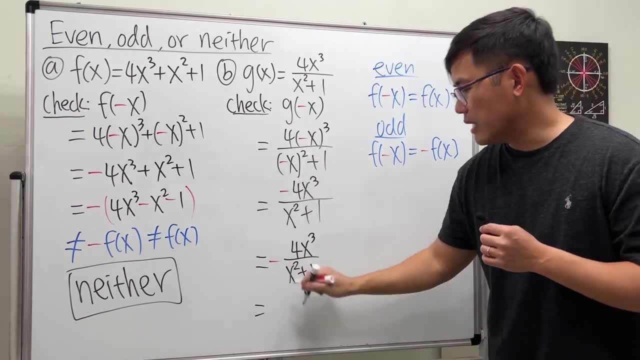 Therefore, we can say: g of negative x is the same as. Therefore, we can say g of negative x is the same as. Therefore, we can say: g of negative x is the same as Negative g of x. Negative g of x. 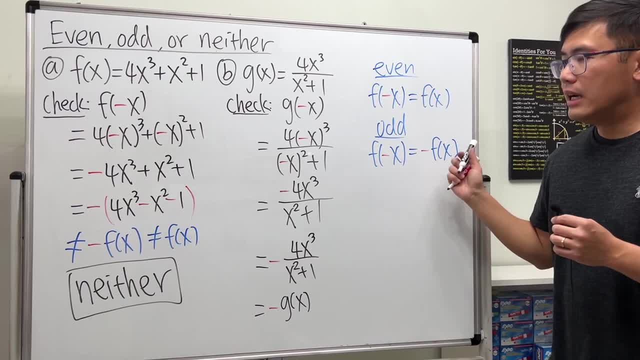 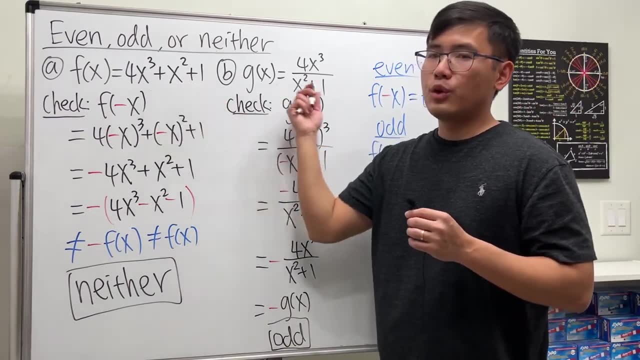 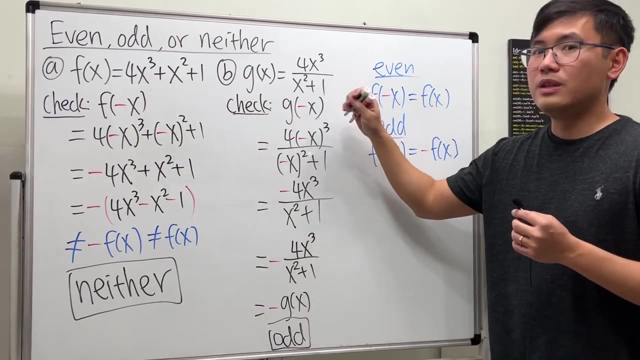 So in this case our function g is actually odd, So this is an odd function. Better yet, just go ahead and graph this and graph that on your graphing calculator. Then you can see that this is not symmetrical about anything and this is symmetrical about the origin. 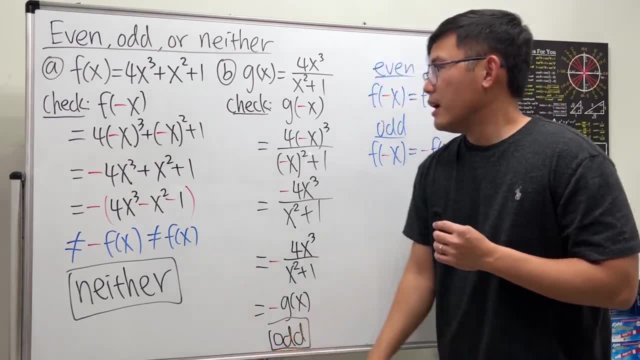 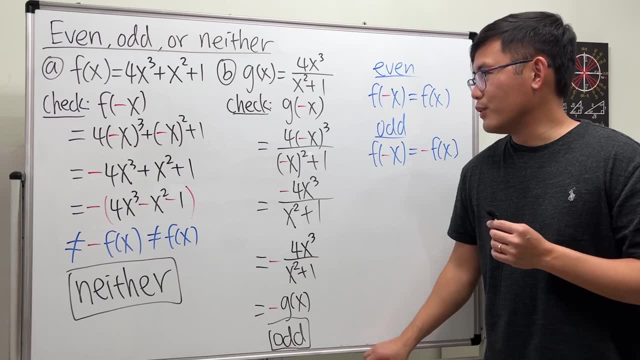 So you can take a look at the graph to be convinced. All right, so that's how you check if a function even or odd or… if not, then neither. before we go, though, i have two questions for you guys. okay, so you try this, right? you will try the following. so why not c and d, right?